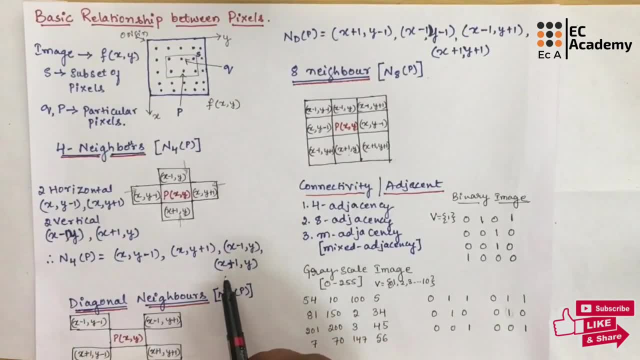 y plus 1, x minus 1 comma y and x plus 1 comma y, so which our four neighborhood pixels. Next, let us understand diagonal neighbors, which can be represented as n d of p. a pixel p with coordinates x comma y has four diagonal neighbors which are connected. 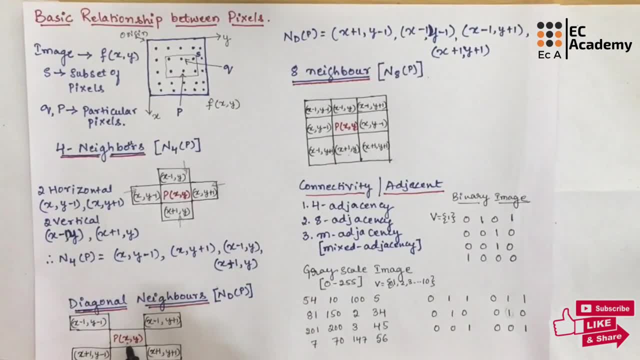 diagonally. So if you consider this pixel, so it is having 4 diagonal neighbors, so which are connected in diagonal form. So here we are having one pixel, one more pixel, another pixel and one more pixel, So 4 pixels in diagonal form. With respect to this pixel, we call 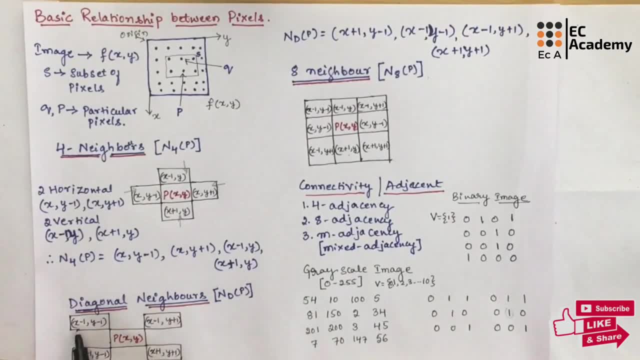 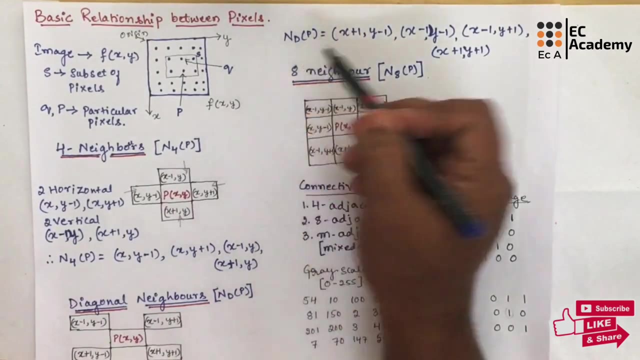 that as diagonal neighbors. So here x minus 1, y minus 1, x minus 1, y plus 1, x plus 1, y plus 1 and x plus 1, y minus 1 forms the diagonal neighborhood pixels. 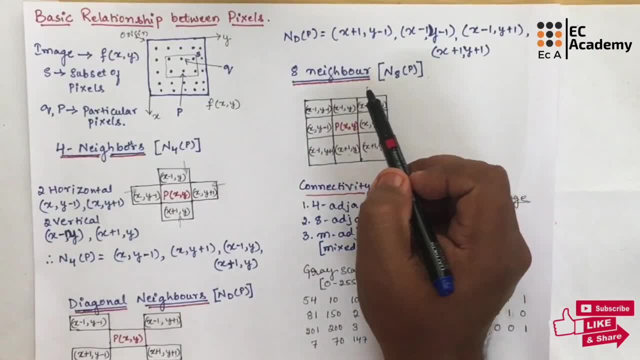 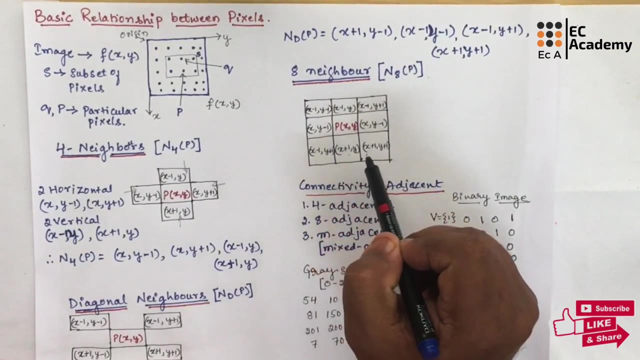 Next we will see 8-neighborhood pixel, or which is also known as 8-neighbors, which can be represented as n8 of p. This is the combination of 4 neighbors And diagonal neighbors. So it is the combination of 4 neighbors and diagonal neighbors. So 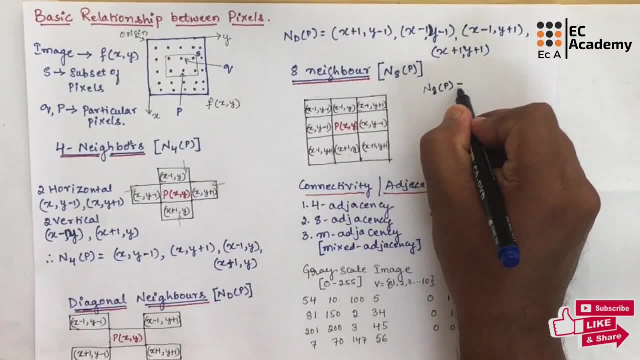 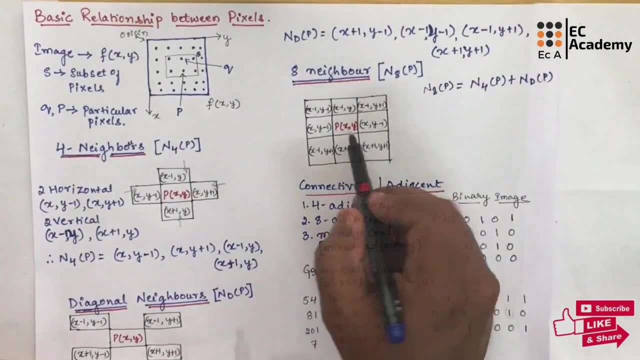 we can say n8 of p will be equal to n4 of p plus nd of p. If we consider the pixel p of x- y, all the surrounding pixels of x- y are 8 neighbors. All are at unit distance from pixel p. 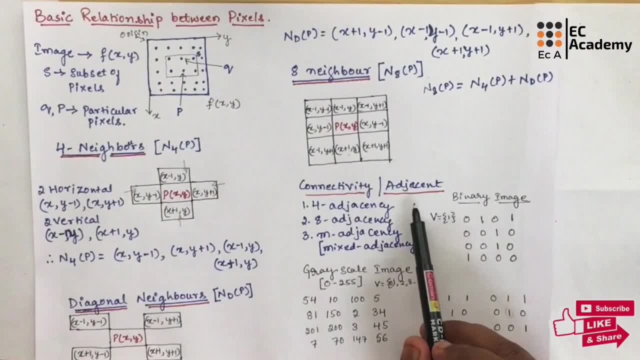 Next we will understand connectivity, or which is also known as adjacent. Connectivity is very important for image processing. There are 3 types of connectivity or adjacent. First one is 4-adjacency, Second one is 8-adjacency And third one is m-adjacency, which is also 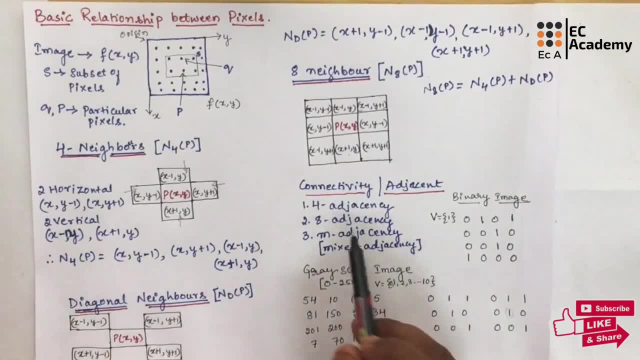 known as mixed adjacency. First let us understand 4-adjacency and 8-adjacency. So first let us consider the binary image: 1-adjacency, 2-adjacency, 3-adjacency, 4-adjacency, 4-adjacency, 4-adjacency, 4-adjacency. 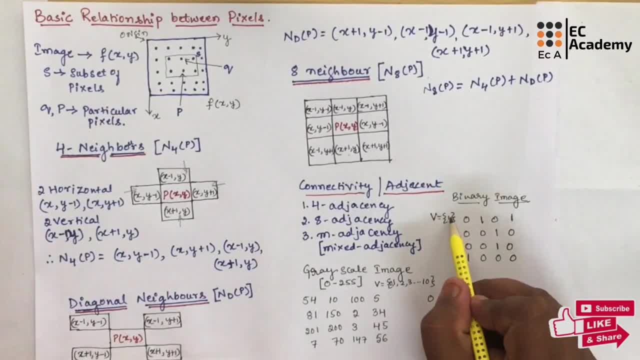 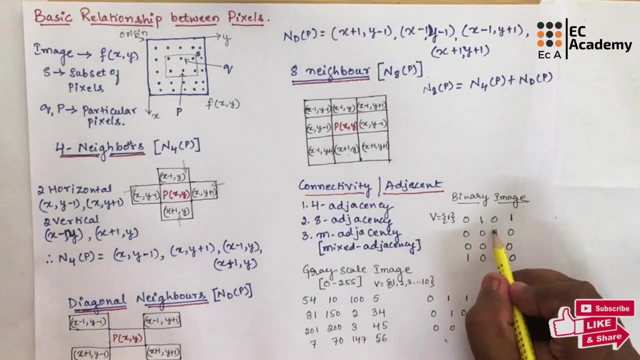 And we will take the set V with value 1, which means we need to concentrate on the value 1 in the image. So binary image consists of both 0s and 1s. Here we are concentrating on the value 1.. If we consider this pixel which is having the value 1, the below pixel, 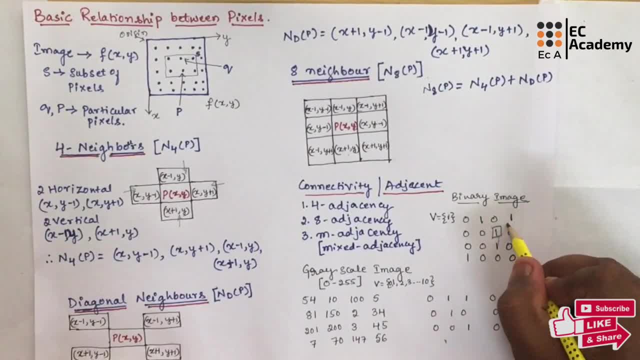 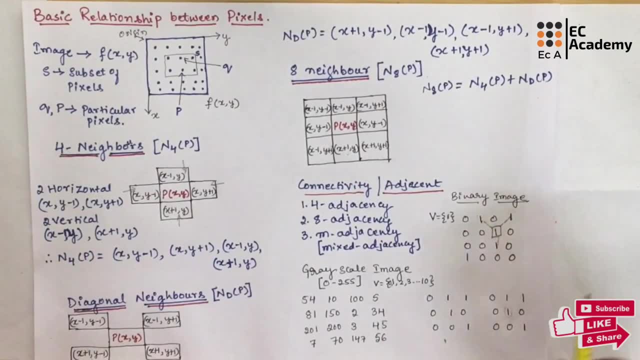 can be connected, And this pixel which is having the value 1 can also be connected. this pixel which is having the value 1 can also be connected. So we can call the connectivity between this pixel and this pixel as 4-way pixel or 4-adjacency, and the connectivity between this. 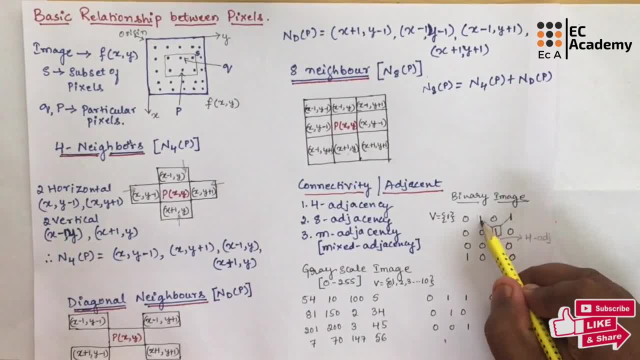 pixel and this pixel and this pixel and this pixel. we can call that as 8-way connected, or it is also known as 8-adjacency. In the same way for grayscale image it will be having the value from 0 to 255 if we take 8-bit value for an image and if we take the 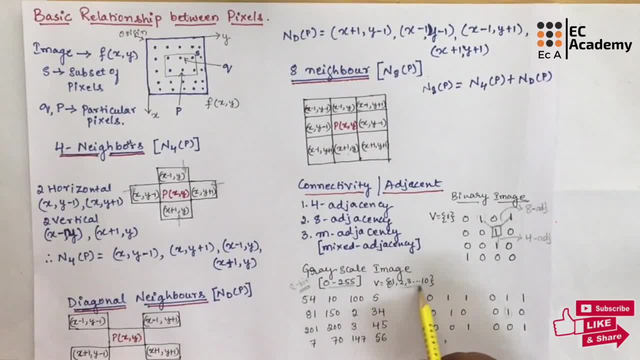 set from 0 to 10.. So these are the values on which we need to concentrate. If we take this pixel, we can connect the below pixel, because the value is between 0 to 10.. We can connect this pixel and we can connect this pixel, So we can call this as: 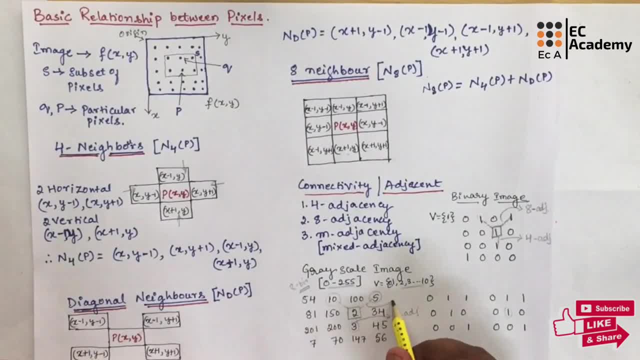 4-adjacency and we can call this as 8-adjacency, because we are connecting in diagonal form. So here we are connecting in a straight line path. that is why it is 4-adjacency. And in this grayscale image, 7 is also between the values 0 and 10, but we cannot connect that to this pixel. 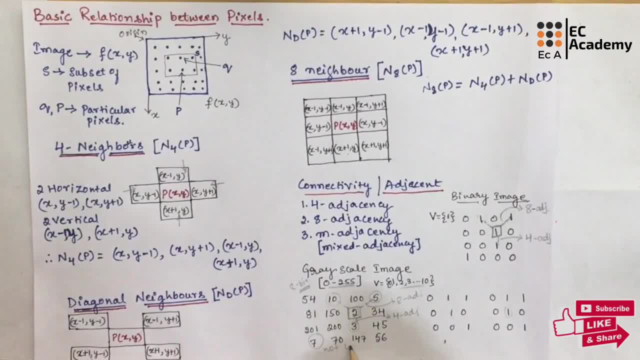 That is why We can say it is not connected. In the same way, for binary image also, this pixel is not connected. So this is about 4-adjacency and 8-adjacency. Next is M-adjacency, which is also known as mixed adjacency.